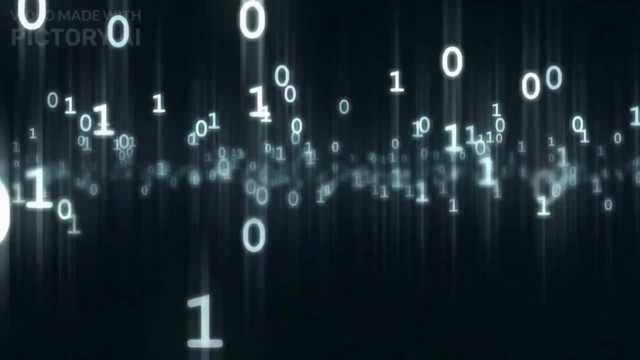 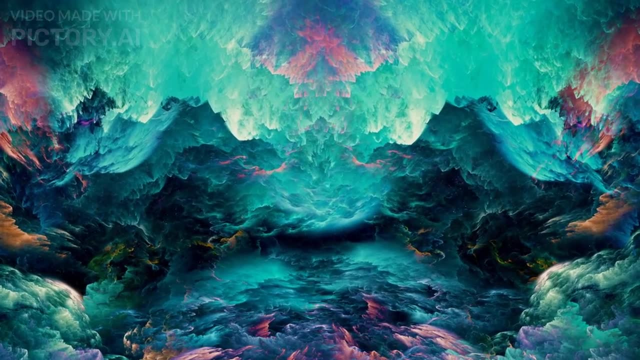 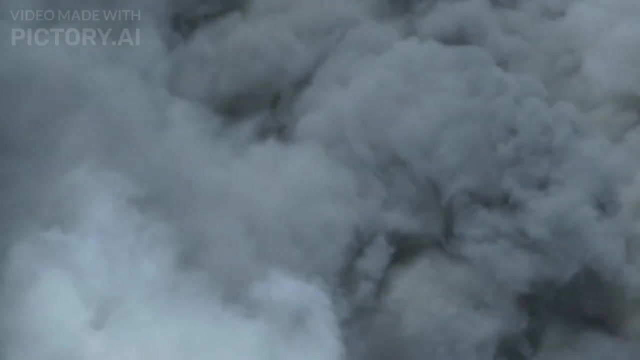 makes use of a number of different systems, But they all depend upon quantum bits or qubits that are in the same quantum state. Most BECs are fabricated from dilute gases of ordinary atoms, But until now a BEC made out of exotic atoms has never been achieved. 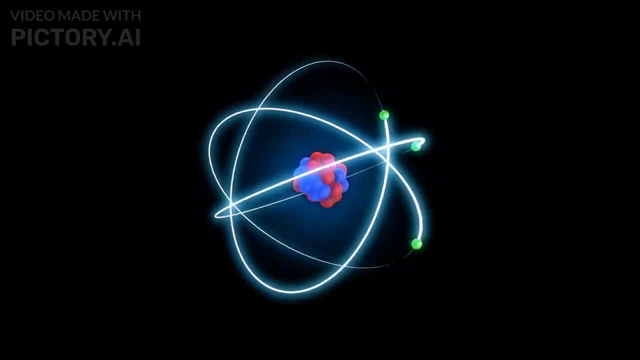 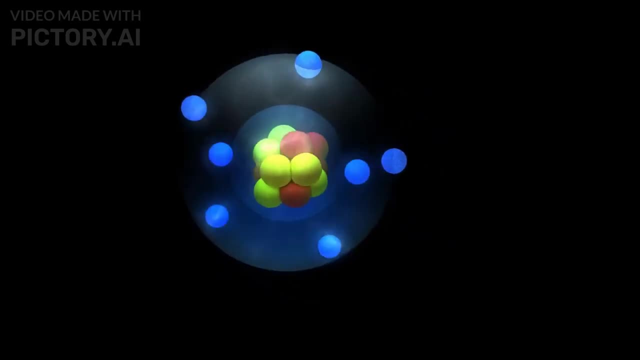 Exotic atoms are atoms in which one subatomic particle, such as an electron or a proton, is placed by another subatomic particle that has the same charge. Positronium, for example, is an exotic atom made of an electron and its positively charged. 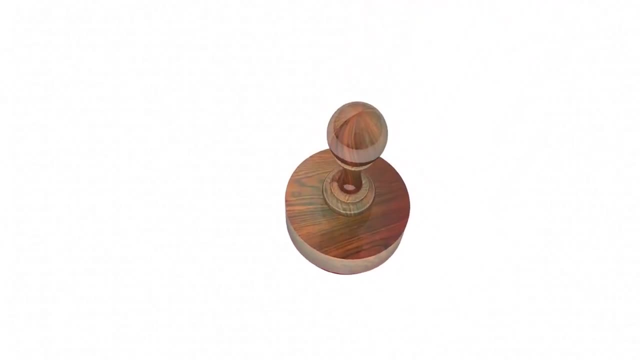 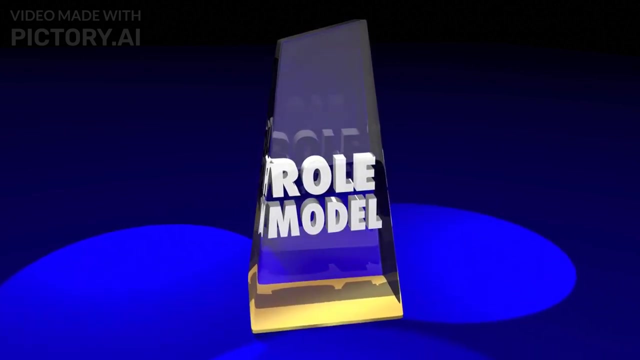 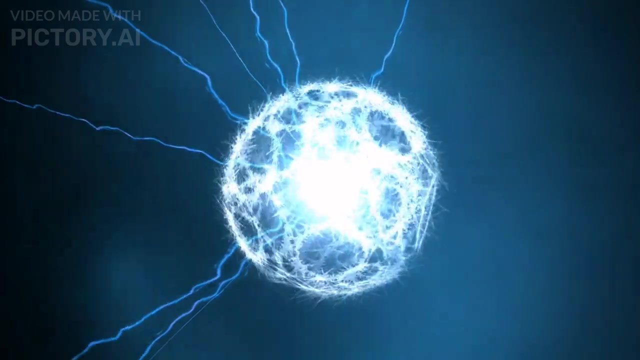 antiparticle, a positron, An exciton is another such example. When light hits a semiconductor, the energy is sufficient to excite electrons to jump up from the valence level of an atom to its conduction level. These excited electrons then flow freely in an electric current. 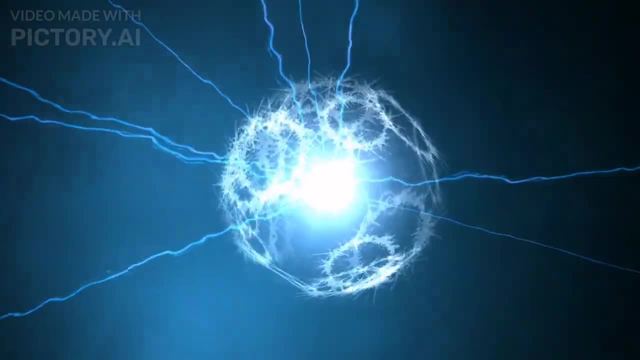 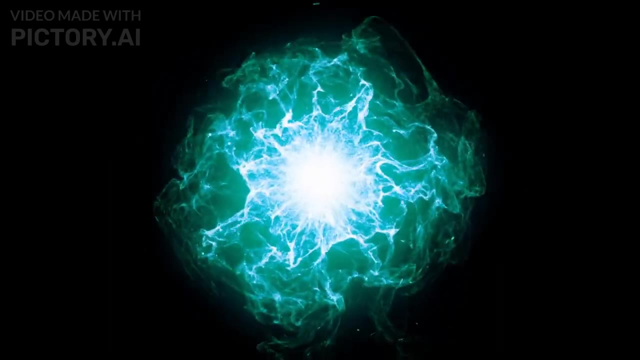 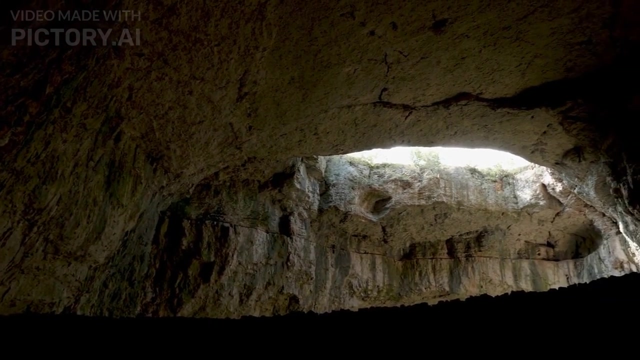 an essence transforming light into electrical energy. When the negatively charged electron performs this jump, the space left behind or hole can be treated as if it were a positively charged particle. The negative electron and positive hole are attracted and thus bound together. 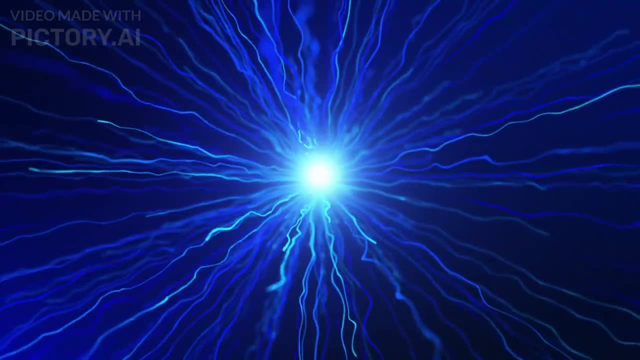 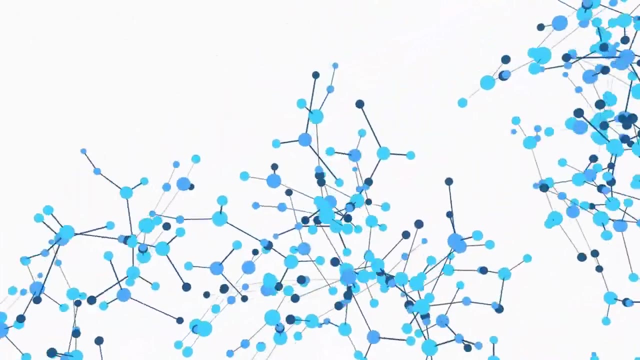 Combined, this electron-hole pair is an electrically neutral quasiparticle called an exciton. A quasiparticle is a particle-like entity that does not count as one of the 17 elementary particles of the standard model. The exciton is an integral of particle physics but that can still have elementary particle. 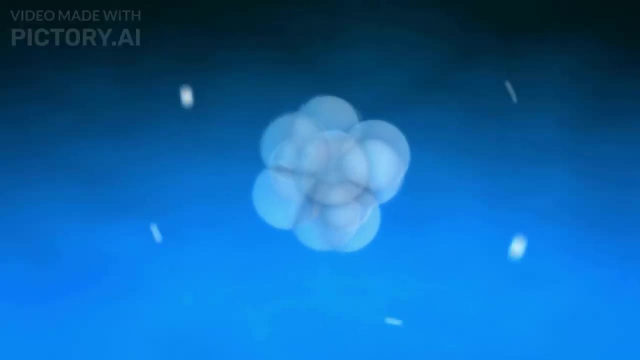 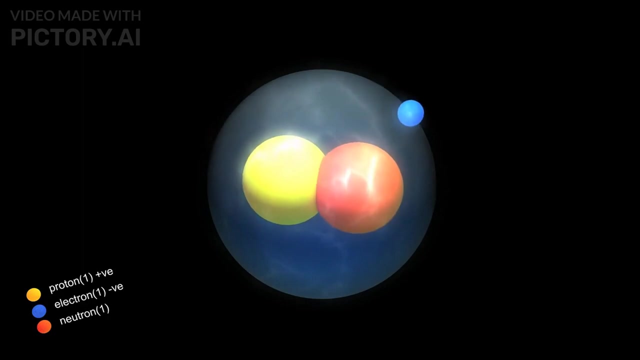 properties like charge and spin. The exciton-quasiparticle can also be described as an exotic atom, because it is in effect a hydrogen atom that has had its single positive proton replaced by a single positive hole. Exitons come in two flavors: ortho-excitons, in which the spin of the electron 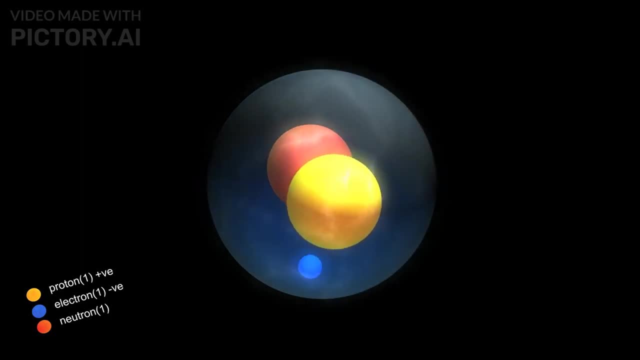 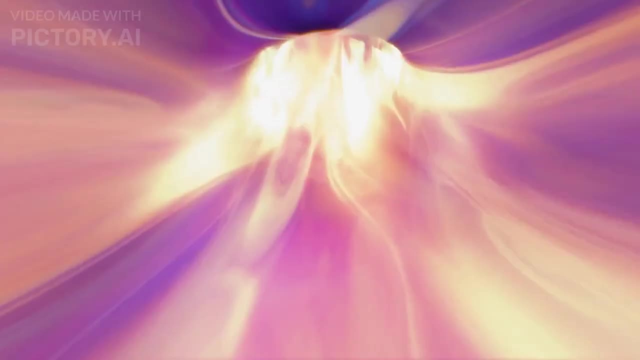 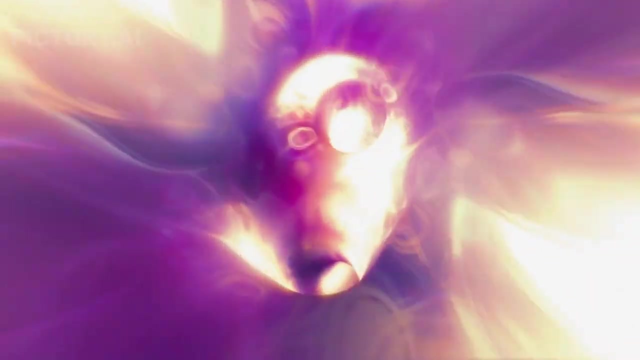 is parallel to the spin of its hole, and peri-excitons, in which the electron spin is anti-parallel- parallel, but in the opposite direction. Electron-hole systems have been used to create other phases of matter, such as electron-hole plasma and even exciton liquid droplets. The researchers wanted to see if they could make 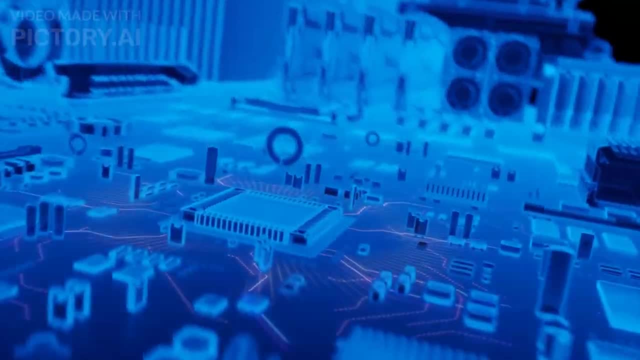 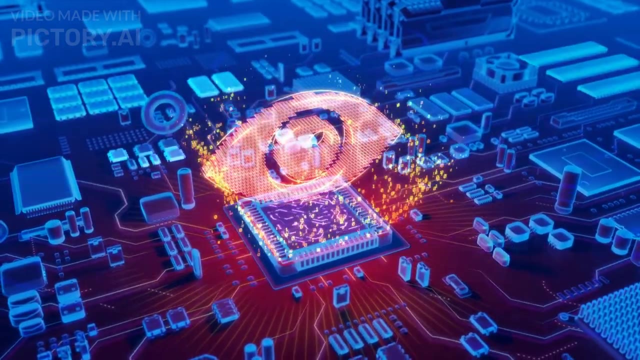 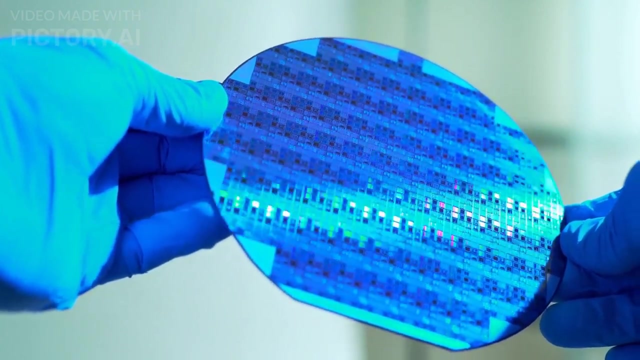 a BEC out of excitons. Direct observation of an exciton condensate in a three-dimensional semiconductor has been highly sought after since it was first theoretically proposed in 1962.. Nobody knew whether quasiparticles could undergo Bose-Einstein condensation in the same way as real particles, said Makoto Kawada-Ganakami, a physicist at 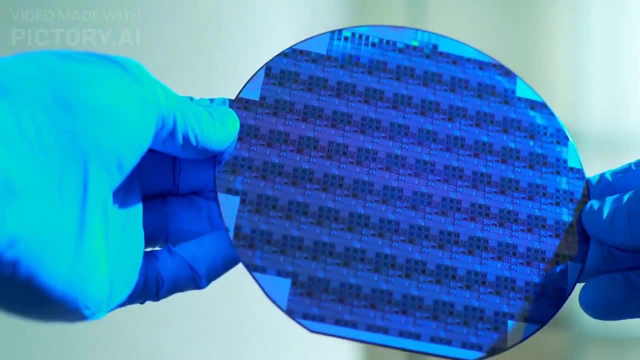 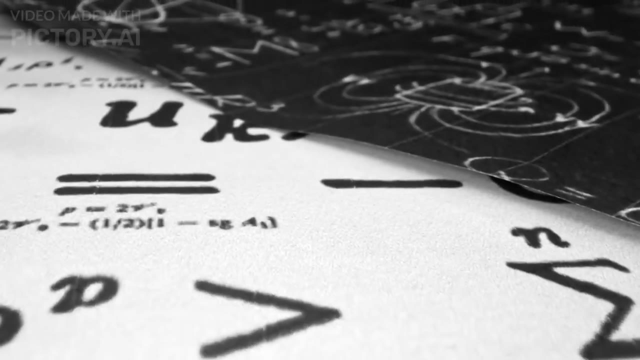 the University of Tokyo and co-author of the paper. It's kind of the holy grail of low-temperature physics. The researchers thought that hydrogen-like peri-excitons created in cuprous oxide, Cu2O, a compound of copper and oxygen, were one. 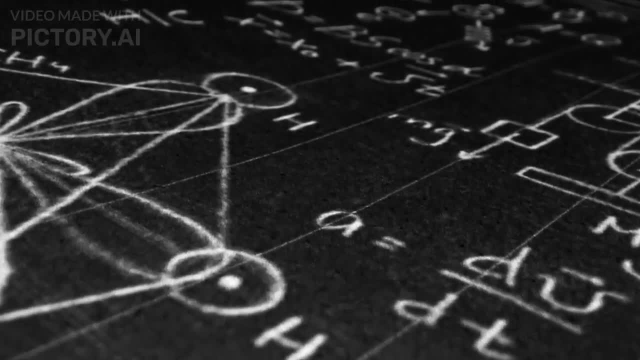 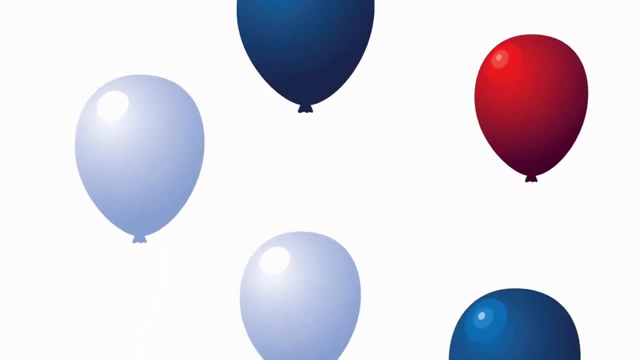 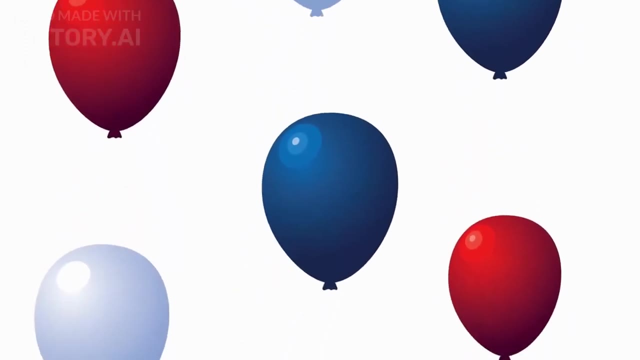 of the most promising candidates for fabricating exciton BECs in a bulk semiconductor because of their long lifetime. Attempts at creating peri-exciton BECs in the form of an exciton condenser have been made in the 1990s, but failed because, in order to create a BEC out of excitons, 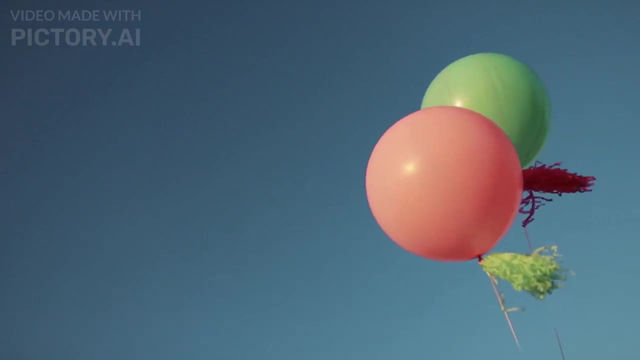 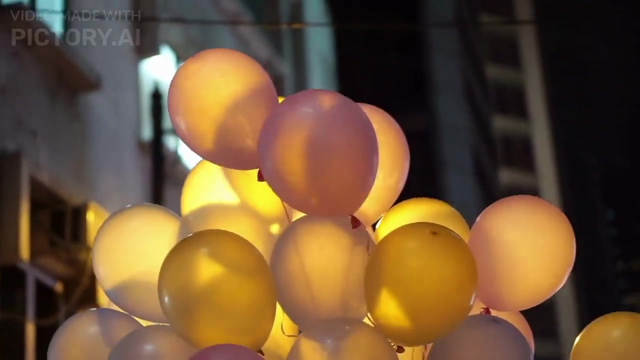 temperatures far lower than that are needed. Ortho-excitons cannot reach such a low temperature as they are too short-lived. Peri-excitons, however, are experimentally well known to have an extremely long lifetime of over several hundred nanoseconds, sufficiently long to. 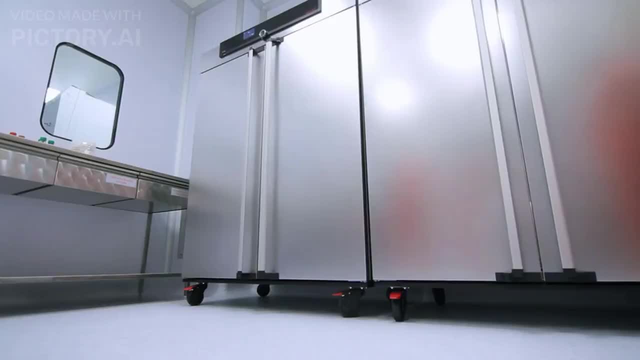 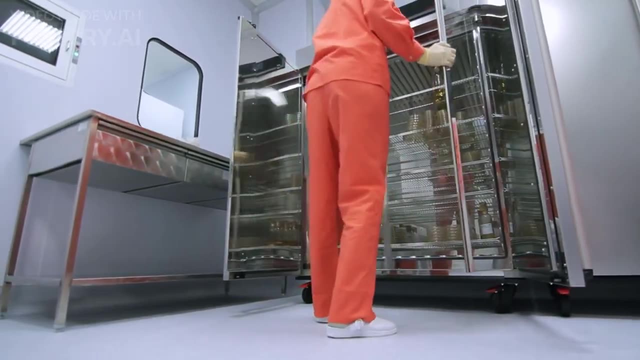 cool them down to the desired temperature of a BEC. The team managed to trap peri-excitons in the bulk of Cu2O below 400 millikelvins using a dilution refrigerator. This is a cryogenic device that cools by mixing two isotopes of. 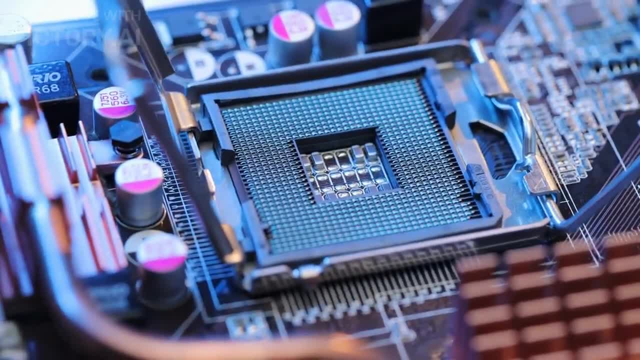 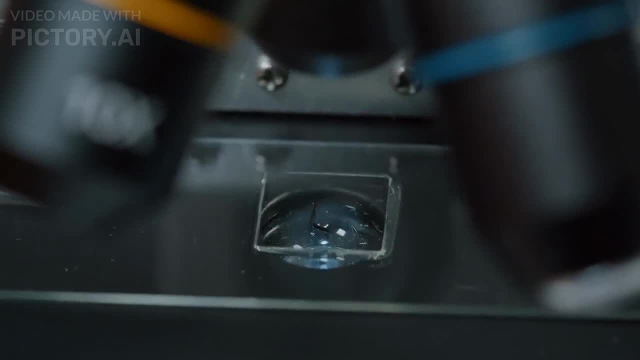 helium together and is commonly used by scientists attempting to realize quantum computers. They then directly visualized the exciton BEC in real space by the use of mid-infrared induced absorption imaging, a type of microscopy making use of light in the middle of the infrared. 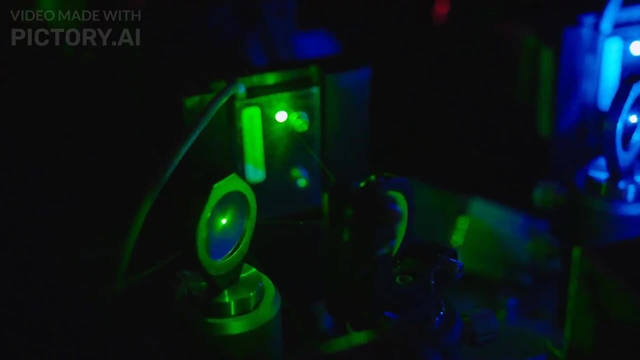 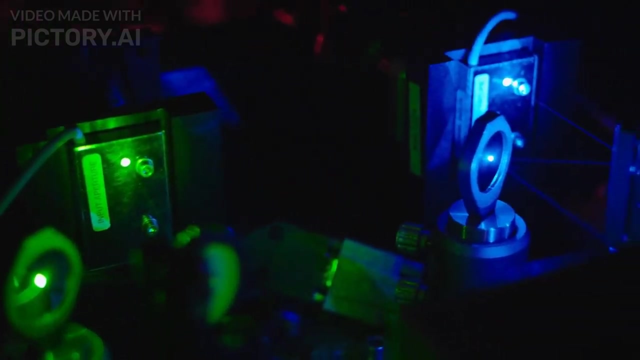 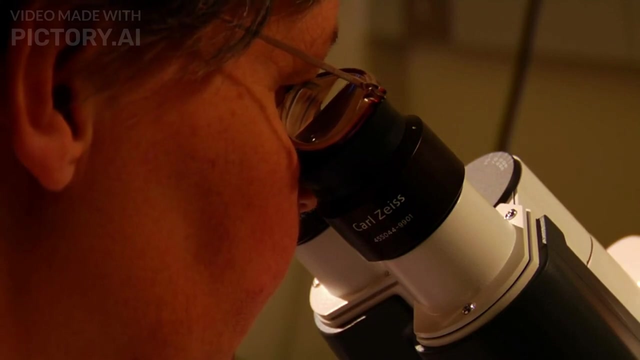 range. This allowed the team to take precision measurements, including the density and temperature of the excitons that, in turn, enabled them to mark out the differences and similarities between exciton BEC and regular atomic BEC. The group's next step will be to investigate the dynamics of how the exciton BEC forms in